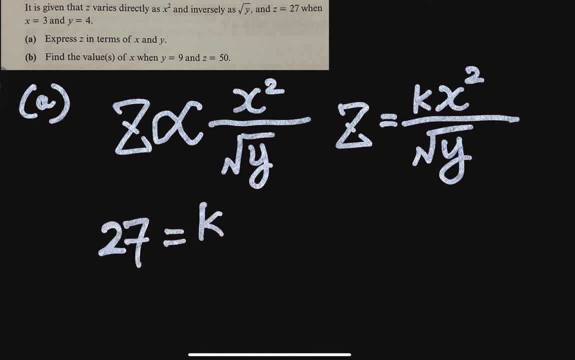 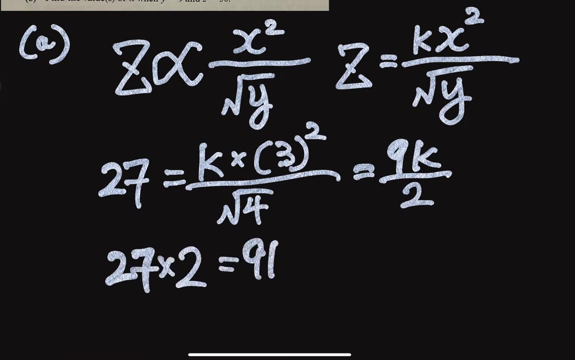 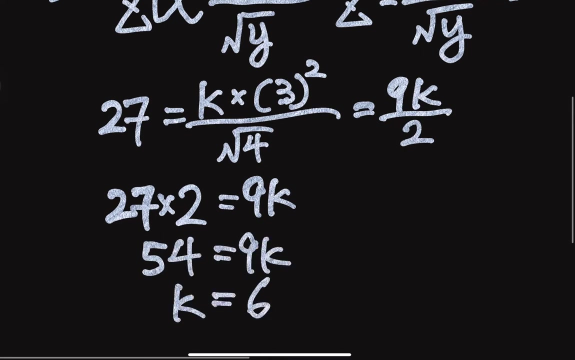 27 will be equal to k times 3.. Therefore, we can see that 27 times 2 will be equal to 9k, And then 54 will be equal to 9k, k will be equal to 6.. Therefore, therefore, we can see that the k here will be 0.. 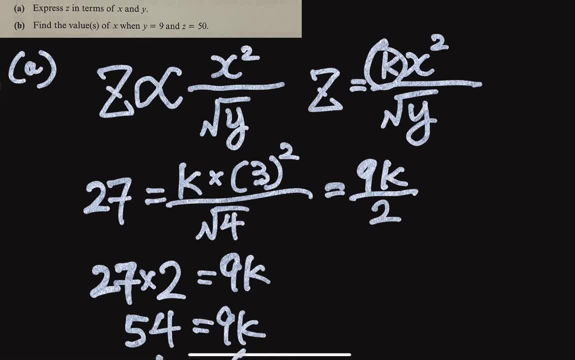 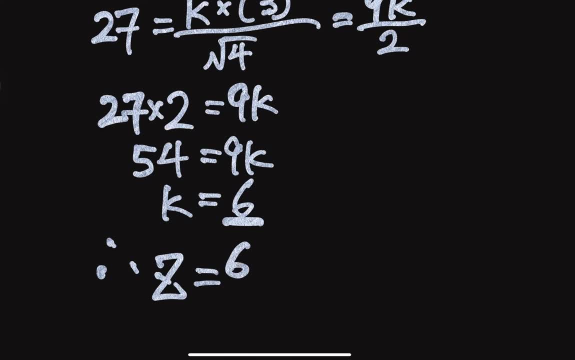 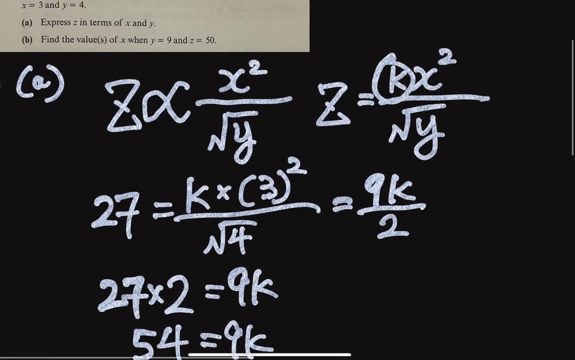 And then we can draw a more beautiful formula for it. Therefore, z, okay, will be equal to 6 times x square divided by y. Okay, so we simply copy this one. Okay, we simply copy this one, And then we input the k here. 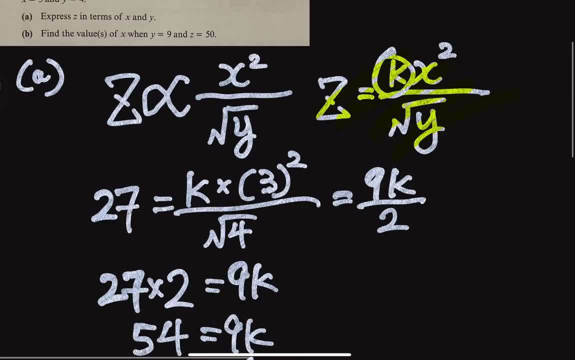 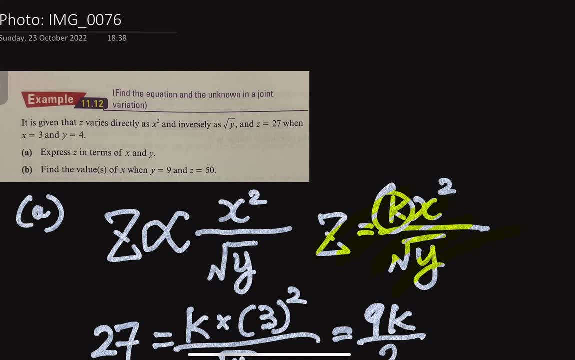 Okay, it will be like that, And then for part b, Part b, It will ask us to find the values of x when y is equal to 9 and z is equal to 15.. So in this case, okay, with reference to our previous answer, 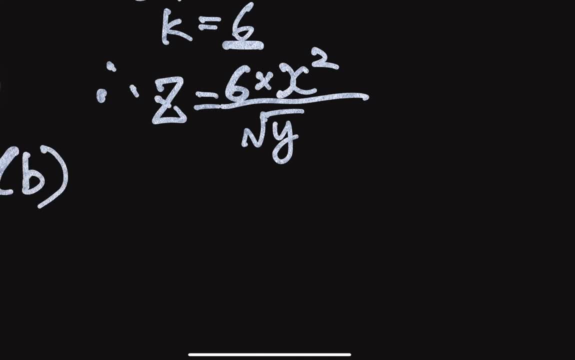 Okay, now we know that the z is equal to 15.. And then we know that 6 times x square, And then it will be 9.. Okay, So in this case, 50, equal to 6 times x square, divided by 3.. 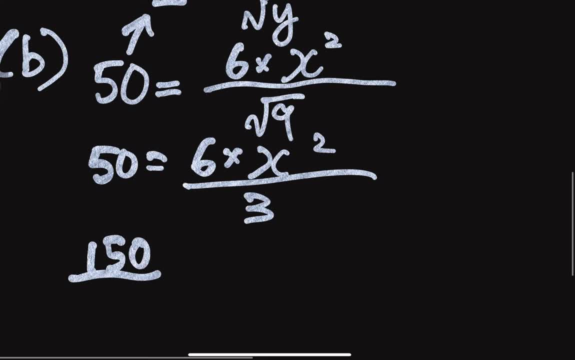 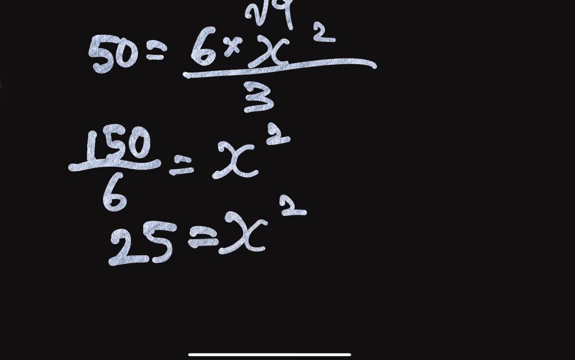 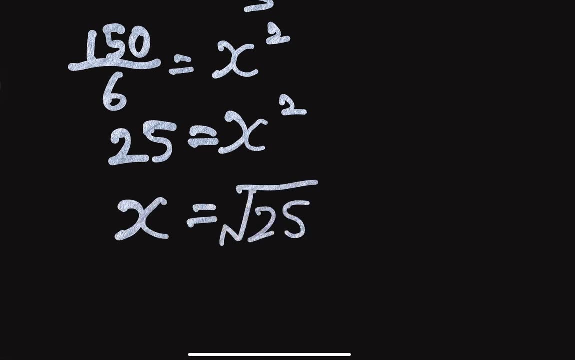 And then, therefore, 150 divided by 6 equal to x square, And therefore 25 equal to x square. So we can see that x- okay- will be equal to the square root of the 25. So x can be equal to 5.. 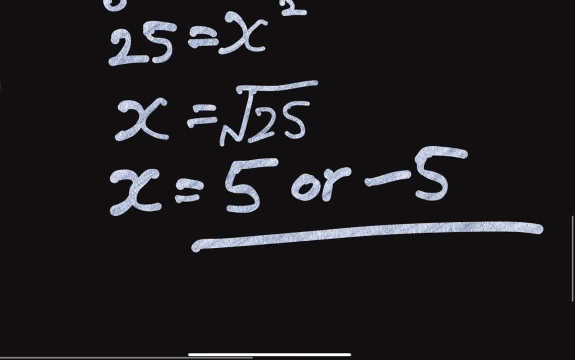 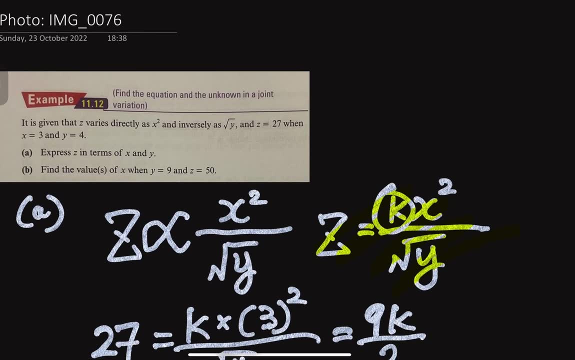 So x can be equal to 5.. Okay, so this is how we solve this question. I hope you guys understand it. If you have any questions, please feel free to leave your comment in the comment section. I will answer and reply all your questions. And please subscribe to my channel. Thank you very much.